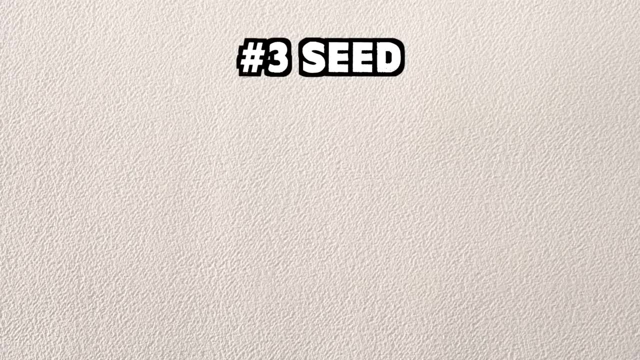 sequences and shots in college basketball history. Three seed has made the national championship 10 times, four of them winning it all. The last three seed to make a title game was Texas Tech in 2019, led by former number six overall pick. 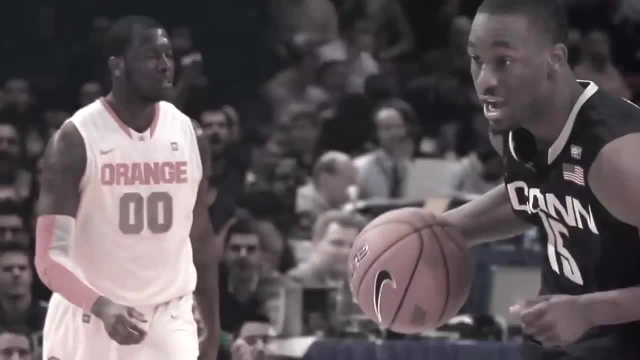 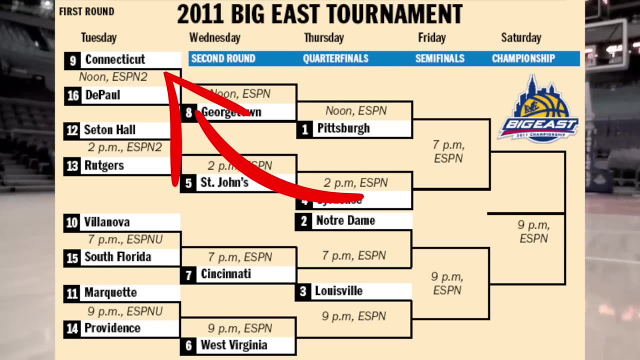 Jarrett Culver, But the last three seed to win it all was the legendary run that took place in 2011 by the UConn Huskies, led by Kemba Walker. Beginning as the ninth seed in the Big East Conference Tournament, UConn went on to win five games in five days, clinching the Big East title. 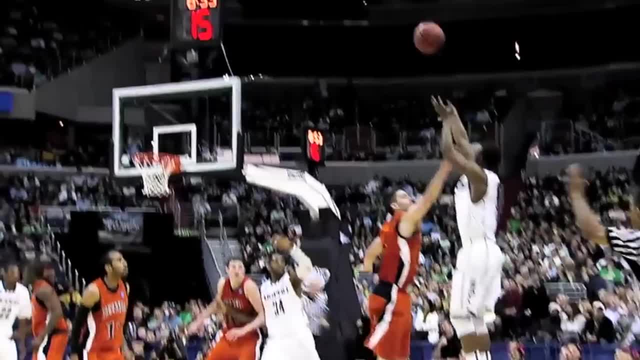 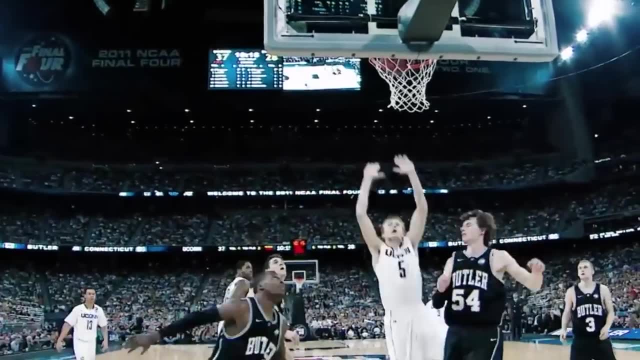 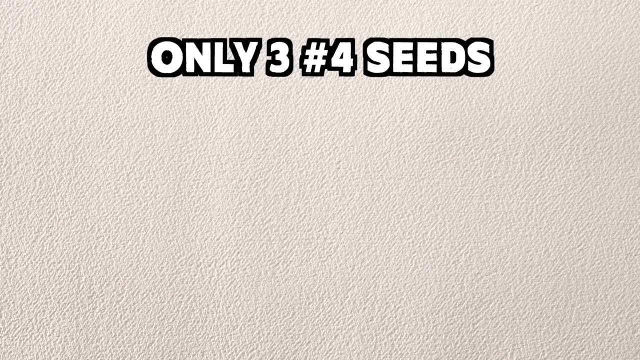 with a Kemba Walker step-back jumper. Then in the NCAA Tournament, as a three seed defeated Bucknell, Cincinnati, San Diego State, Arizona, Kentucky and finally Butler to their championship trophy. Truly one of the best stories ever And runs we've seen from a team in recent history Only three number four seeds have. 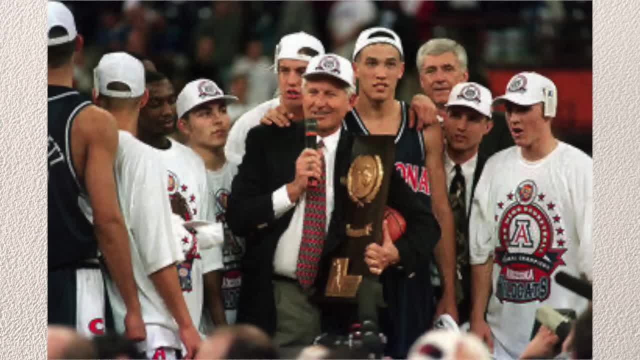 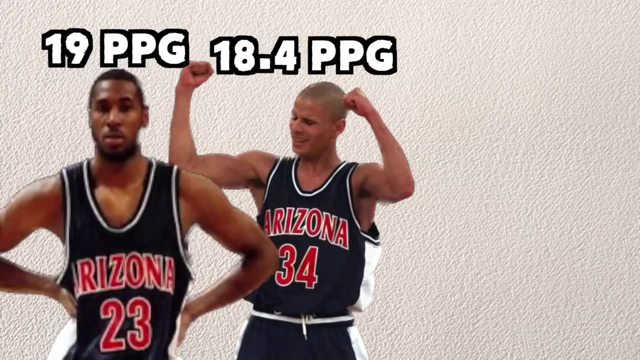 ever made a title game in the NCAA Tournament, with the 1997 Arizona Wildcats being the only ones to ever win. This team actually was really good. They had Michael Dickerson, who averaged 19, to game Miles Simon 18.4,. Mike Bibby 13.5,. Jason Terry 10.5.. It's truly not. 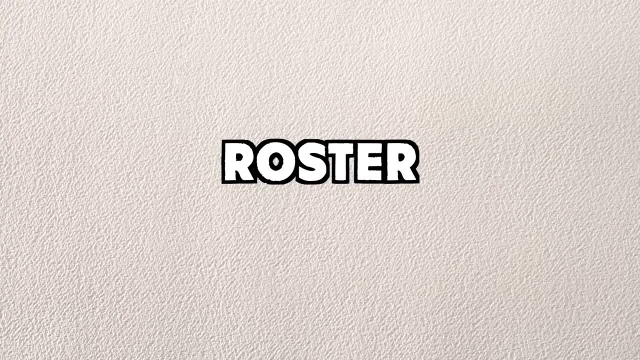 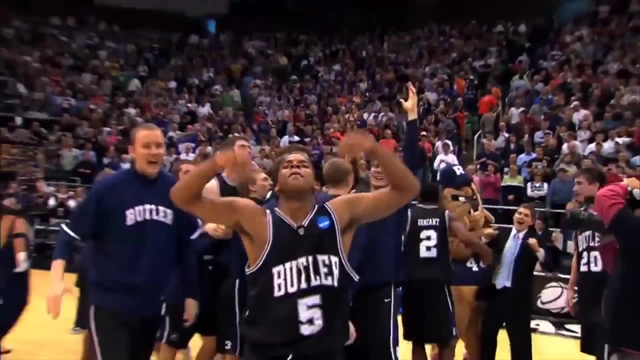 surprising that they're the only four seed to ever win it, because that's a really talented roster And a five seed has never won the national title. finishing as the runner-up three times in tournament history, The 2010 Butler Bulldogs came the closest to succeeding, losing in absolute dramatic fashion. 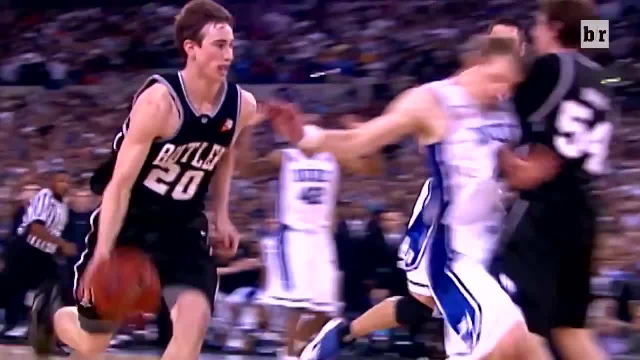 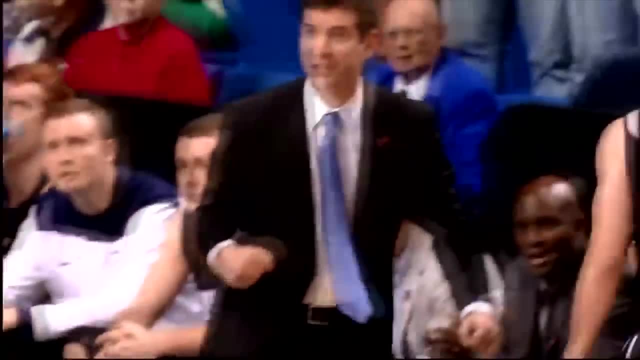 61 to 59, after Gordon Hayward almost hit a half-court buzzer beater to win. That Butler team was loaded with Gordon Hayward, Shelvin Mack, Matt Howard, coached by Brad Stevens. I remember as a kid cheering for them so hard, wanting them to win, and just being crushed when Gordon Hayward's shot. 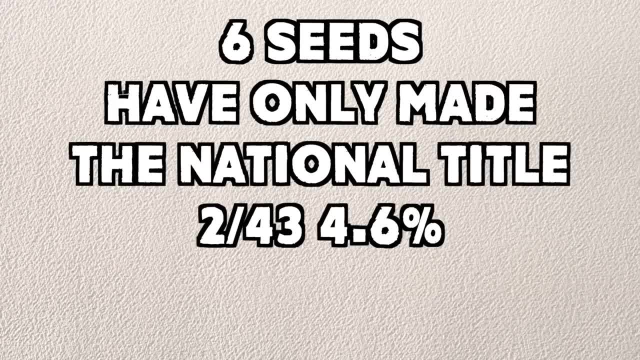 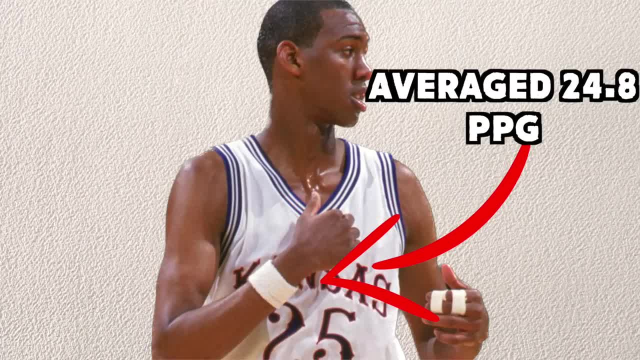 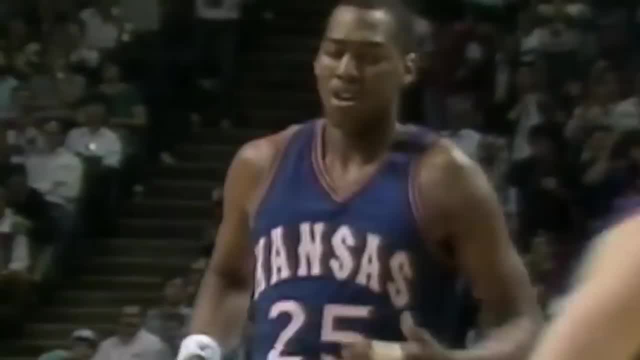 was just a bit off the mark. Six seeds have only made the national title twice and won it once, which was Kansas in 1988.. This was Danny and the Miracles, led by senior forward Danny Manning. Manning was an absolute stud as a senior, averaging 24.8 points per game. He was also named the Naismith College Basketball. 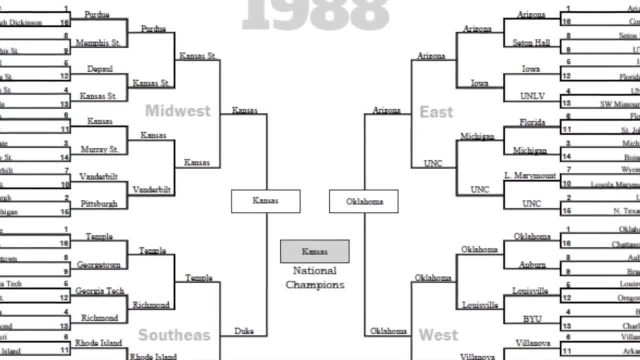 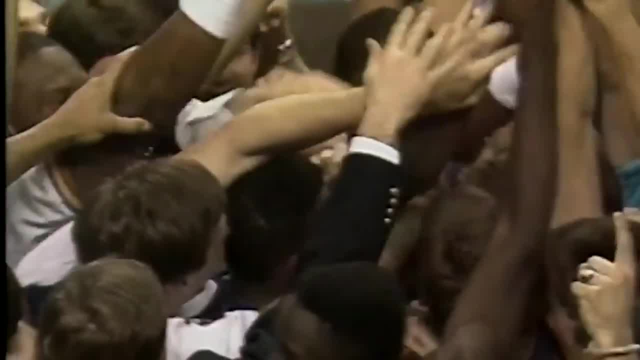 Player of the Year, But all we'll go into here is that they ended up playing Oklahoma in the national title, a team they had lost two times, defeating them 83 to 79. This team truly does deserve its own video. A seven seed in the NCAA tournament has only appeared in the national title. 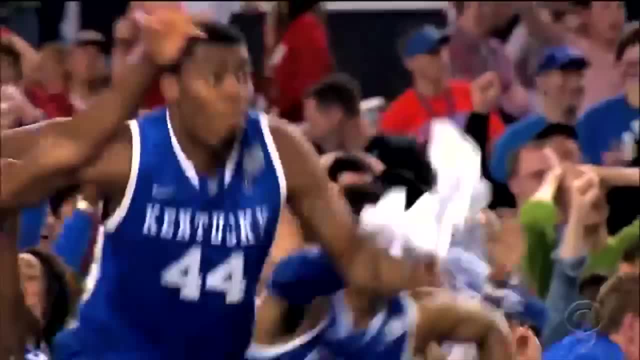 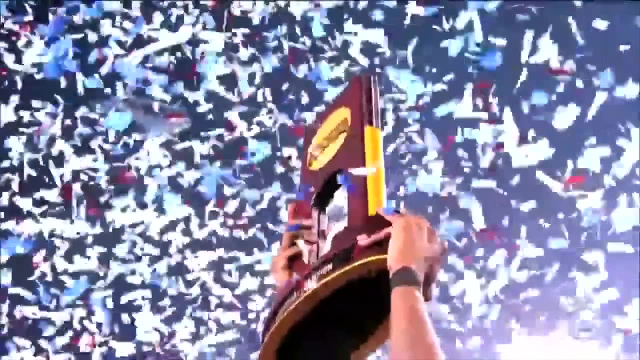 once, and that was the University of Connecticut in 2014,, where they beat the National League of Kentucky, making them not only the only seven seed to make a national title, but to win a national title. Coached by Kevin Olley, who was just succeeding Jim Calhoun, this team was also 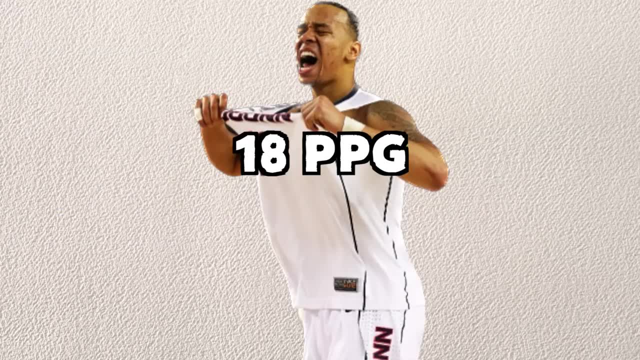 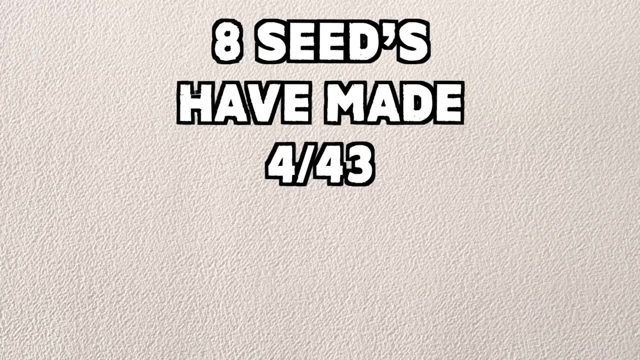 banned from postseason play. the year before Shabazz Napier kind of carried this team to a national title, making it UConn's second national title in four seasons. Eight seeds have made four appearances in national title games, with the most recent one being last year's North Carolina team. 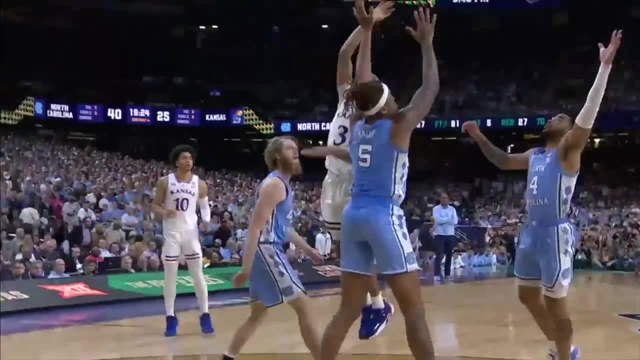 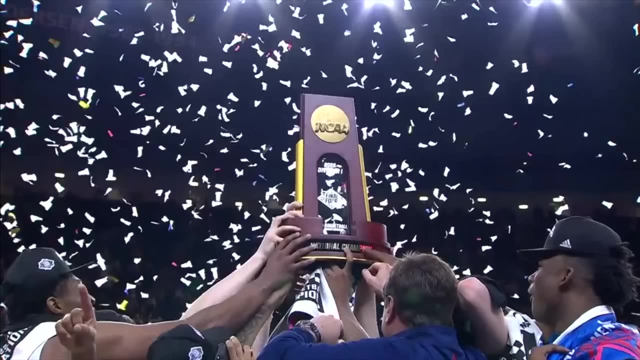 This was a team that just got hot at the right time But ended up running into a very talented Kansas team led by Ochai Akbaje. There has, however, been one eight seed to win it all in tournament history back in 1985, and that was the Villanova. 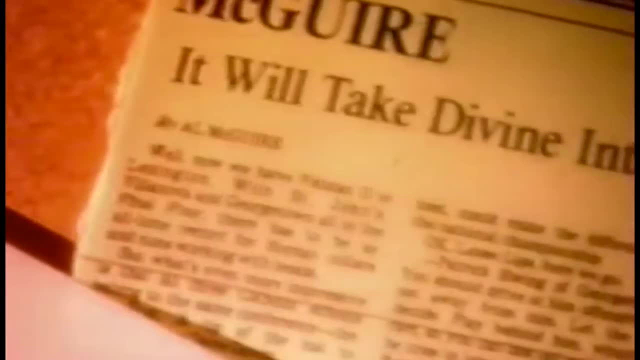 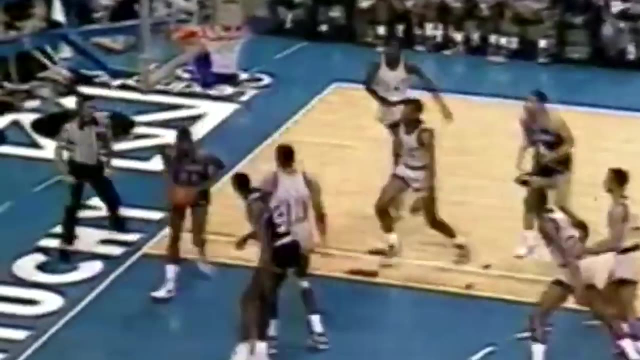 Wildcats In a game that was considered one of the biggest upsets in NCAA history. Villanova shot 79% from the field, going 22 of 28 and 9 of 10. in the second half, They defeated the Patrick Ewing. team. they had lost to twice in the regular season and this marks the lowest seed to ever win an NCAA championship. Unfortunately for the nine seed, a final four is the furthest one has ever made it and it's only been one team, the 2013 Wichita State Shockers. One of the more popular final. 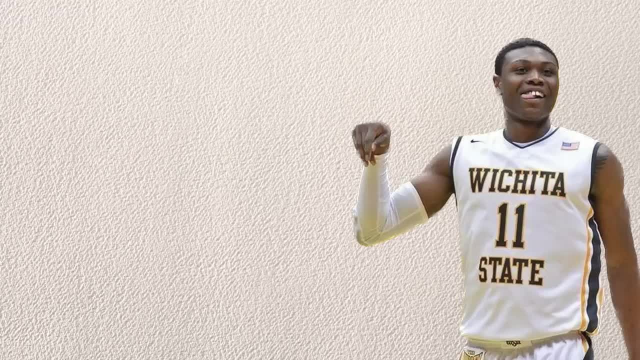 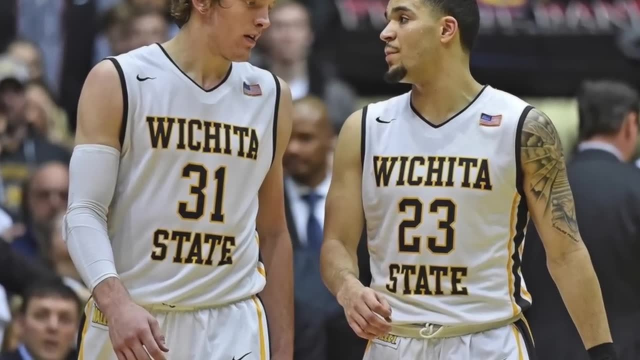 four runs in recent memory. this team was led by Cle Anthony Early, Malcolm Armstead and Carl Hall. While Fred VanVleet and Ron Baker were on the team and were definitely contributors, they were not as much of a contributor as they were in the following season when Wichita State was 35 and 1,. 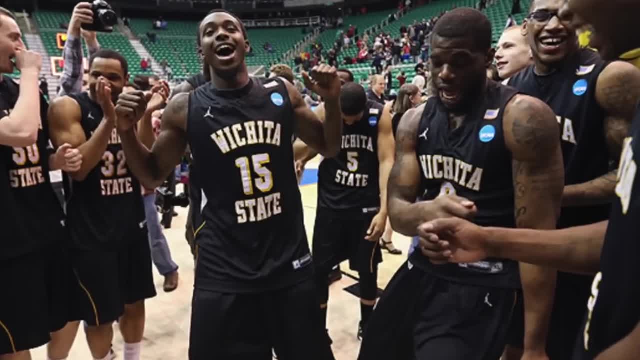 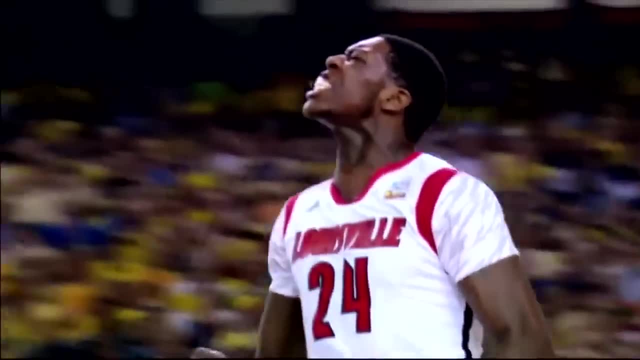 but only made the sweet 16.. The 2013 squad that made the final four upset Gonzaga with Kelly Olynyk in the second round, before falling 72 to 68 to a Louisville team, a team that ended up winning the national title that year. As far as 10 seeds go, the furthest one has ever made. it was the final. 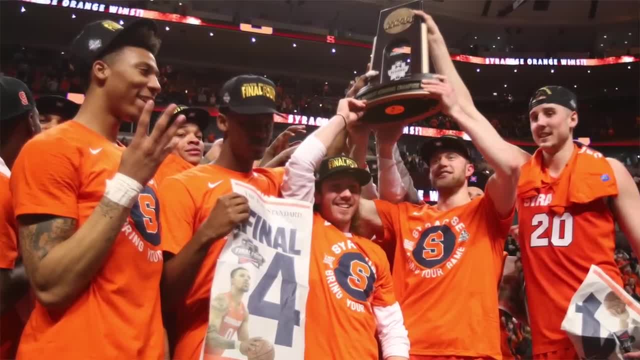 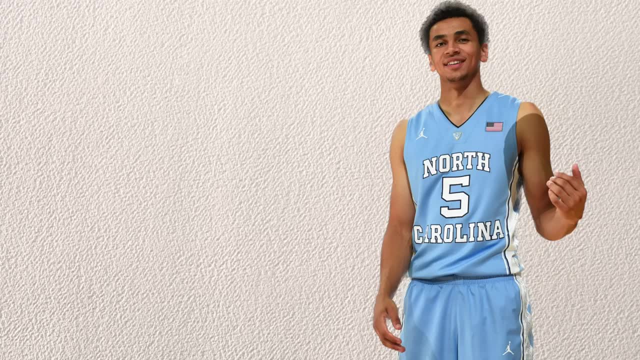 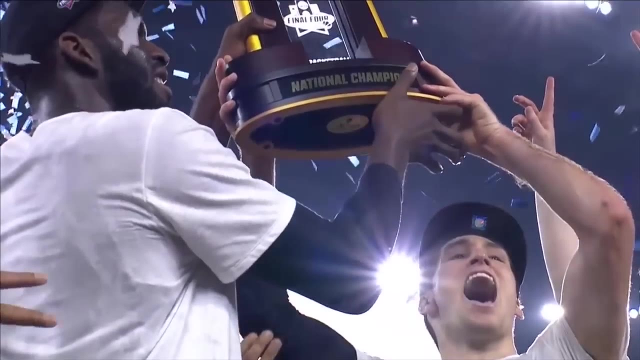 four, and that was in 2016,. the Syracuse Orange: This was a team that most bracketologists didn't even have in the tournament field. Fortunately, this remarkable run was ended by Marcus Page and the North Carolina Tar Heels, a team that ended up falling to the 2016 Villanova Wildcats, which we talked about earlier in the 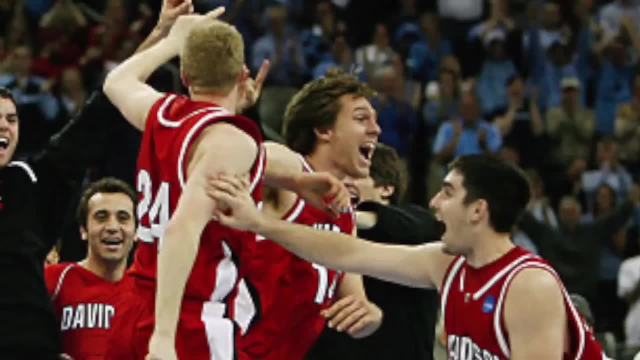 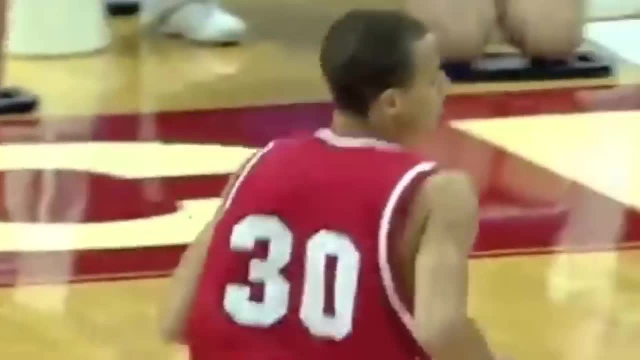 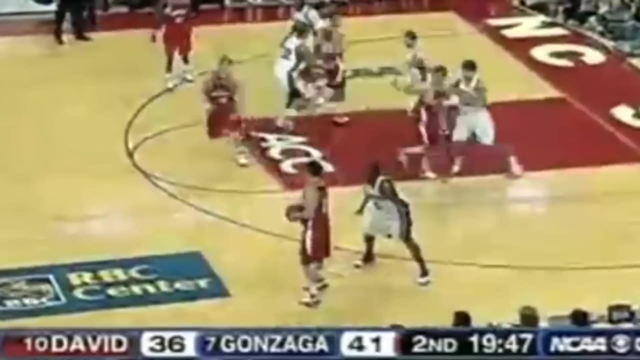 video. But let's get to the fun 10 seed everyone wants to talk about, and that's the 2008 Davidson Wildcats, led by baby-faced Stephen Curry. Stephen Curry was practically a nobody coming into this NCAA tournament. He was putting up great numbers, averaging 25.9 points per game In the first round. 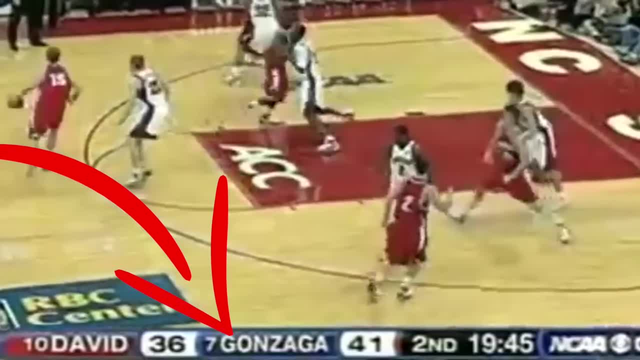 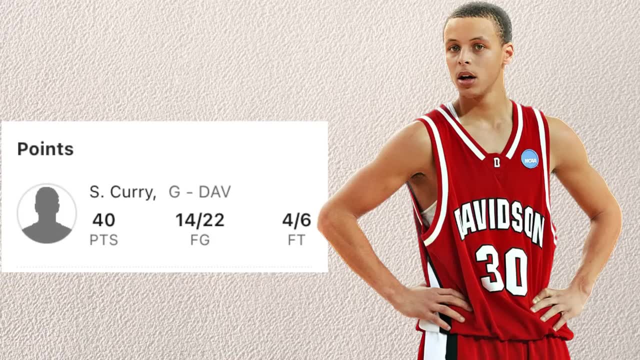 Davidson found themselves down five at half. a seven seeded Gonzaga before Stephen Curry went off for 30 in the second half, winning 82 to 76.. Steph ended the game with 40.. In the second round of the tournament they played Georgetown again. 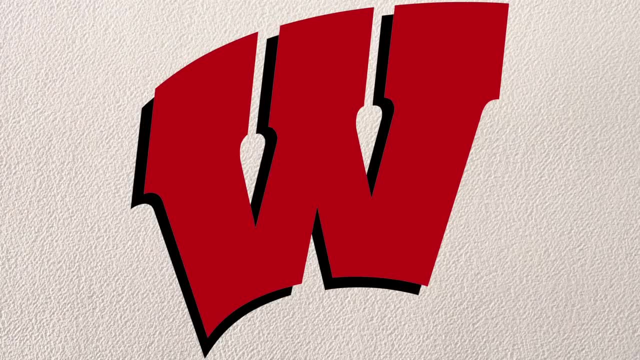 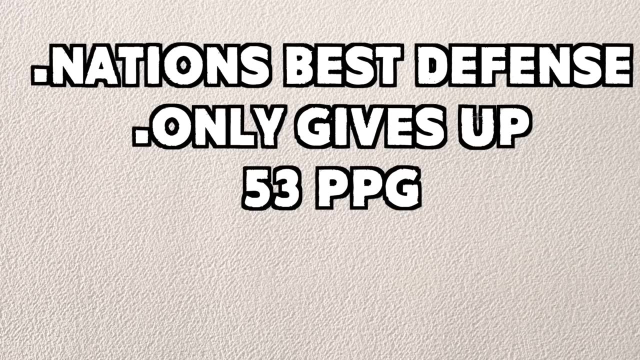 Stephen Curry led a comeback victory, matching up against a third seeded Wisconsin Badgers in the Sweet 16.. This team was the nation's best defense and they only gave up 53 points per game. Stephen Curry had 33 points himself, punching their ticket to the Elite Eight, Unfortunately. 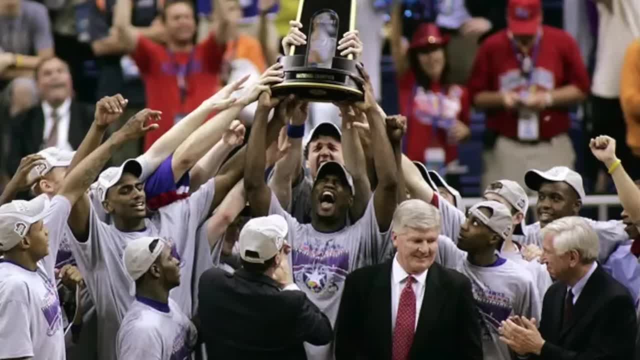 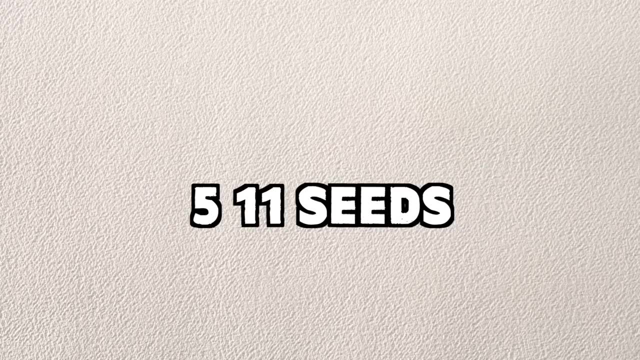 Stephen Company ran into the eventual national championship. Stephen Curry was the only team that turned out to be a champion in the Kansas Jayhawks. To me, this was the greatest single-player run in NCAA history. Somehow there have been five 11 seeds in the history of the NCAA tournament that. 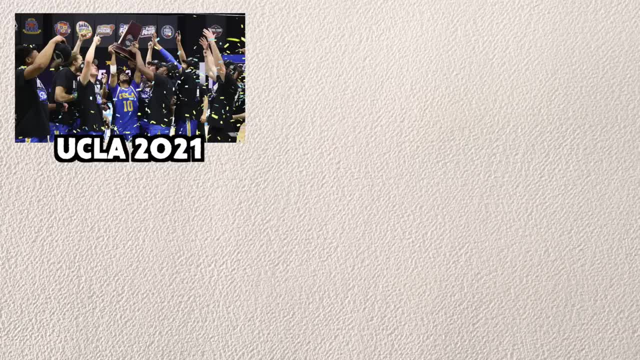 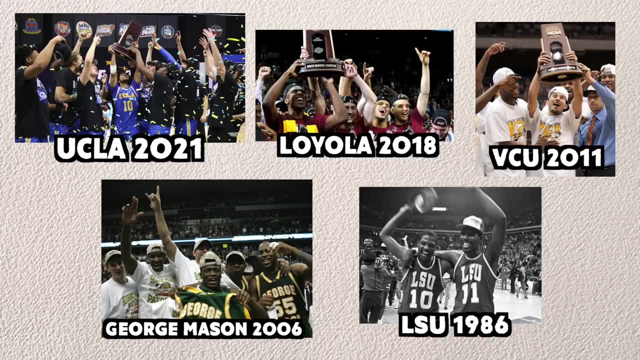 have made it to the Final Four, including UCLA in 2021, Loyola Chicago in 2018, VCU in 2011,, George Mason in 2006, and LSU in 1986.. And as much as I'd love to talk about each one of these teams, 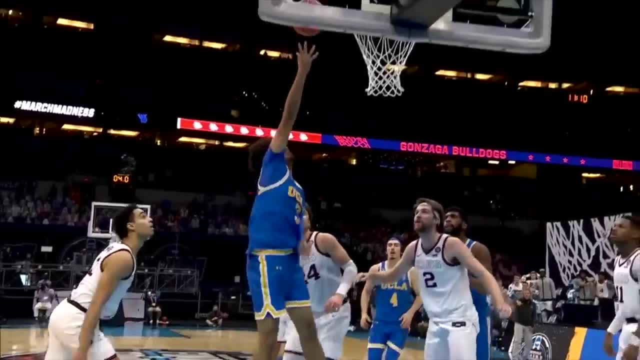 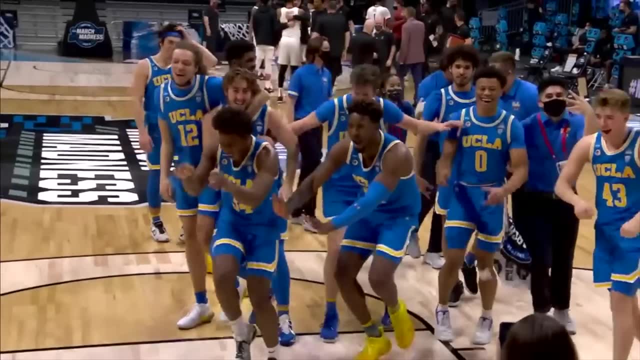 because these runs were incredible. the one that sticks out to me was the most recent one: UCLA in 2021.. Beginning in the first four and finishing in the Final Four. I'd love to talk about every single game individually, but let's focus on this Final Four game against a Jalen Suggs-led Gonzaga. 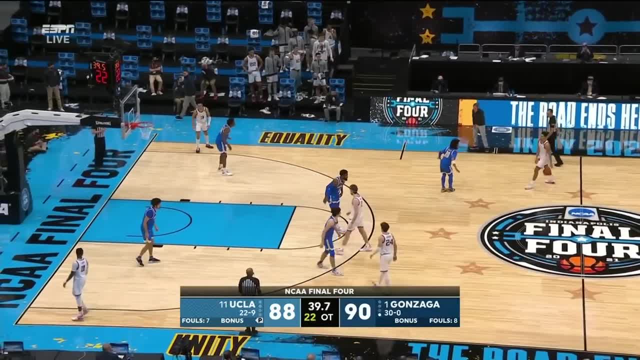 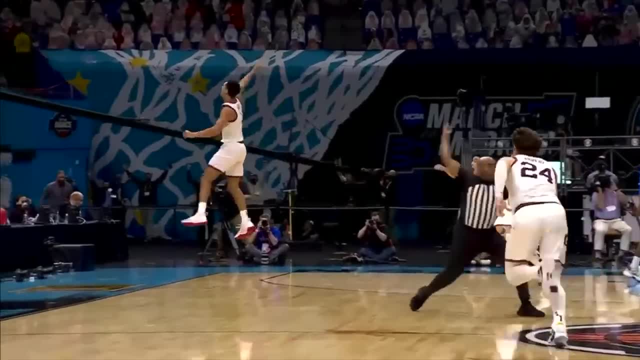 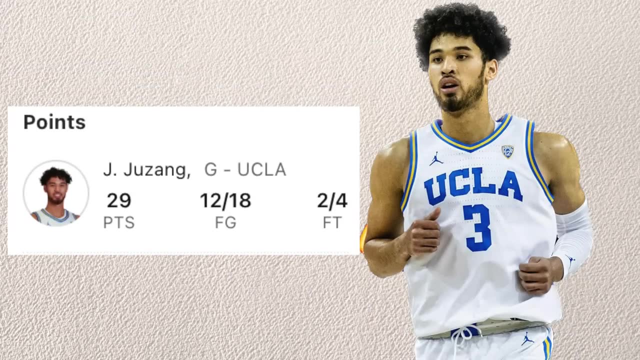 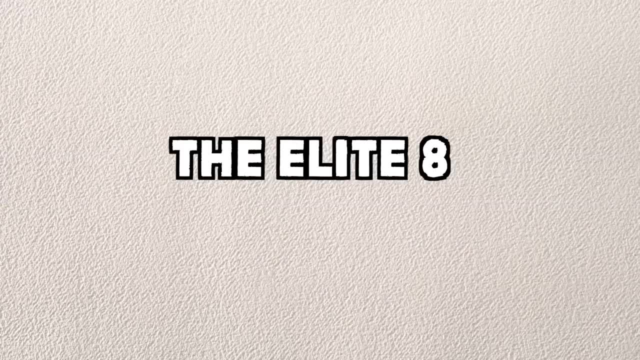 where, all in all, Grandash and LeS Austin beat the SEC, Diwow in the Final Four. In fact, this return wasn't entirely support for the巫, seeing a plus five lead like a has ever made the elite eight, and that's a 2002 missouri tigers team beating all of their teams. 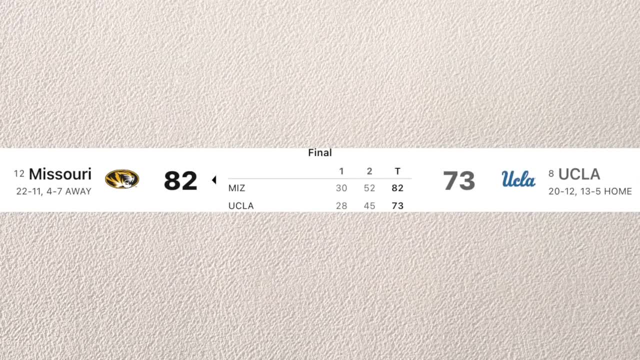 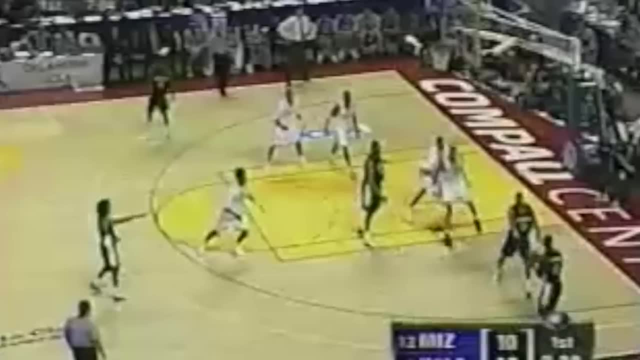 by almost double digits, including a nine point win against ucla in the sweet 16. the tigers lost to oklahoma in the elite eight 81 to 75. i'm still shocked that we haven't seen more 12 seeds make it to the elite eight, the furthest a 13 seed has ever made it as the sweet 16, which has happened. six. 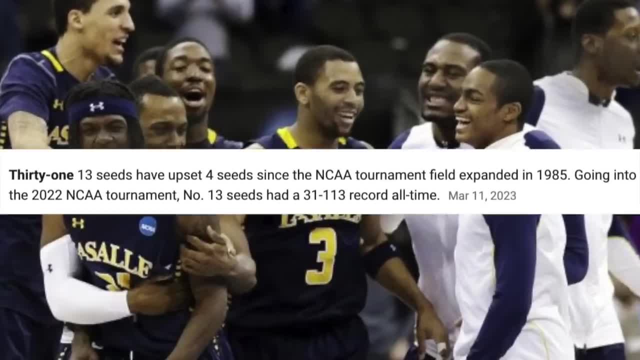 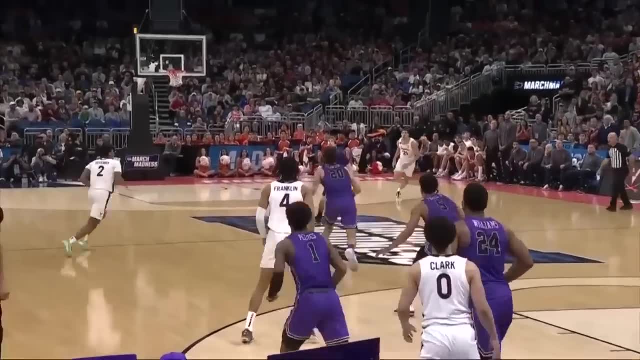 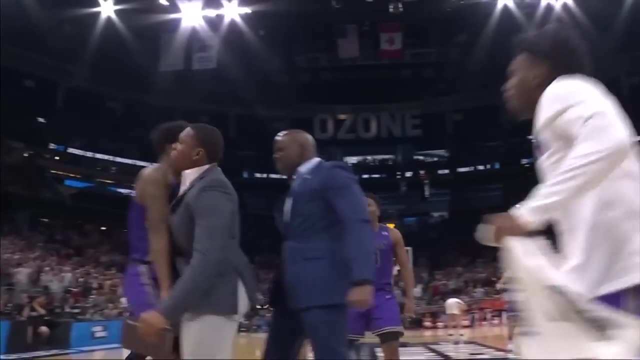 times, the latest one being lasalle in 2013, but we have seen a 13 upset of four almost every year of the last 37 ncaa tournaments, including this year, when the firman paladins beat the virginia cavaliers, and one of the craziest last second turnovers that i've seen in recent memory. we've 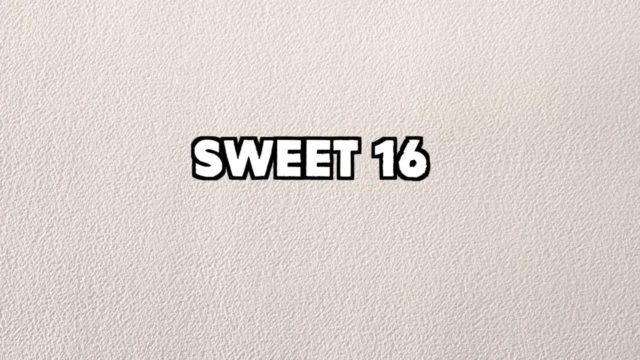 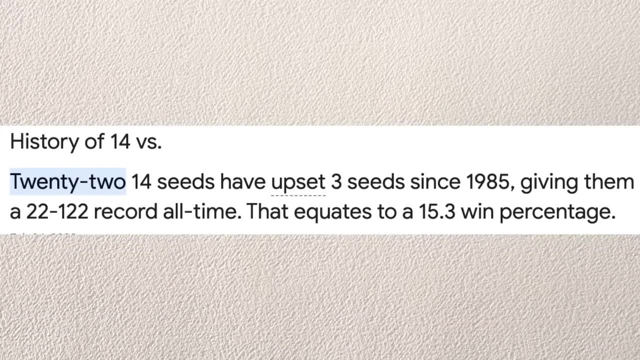 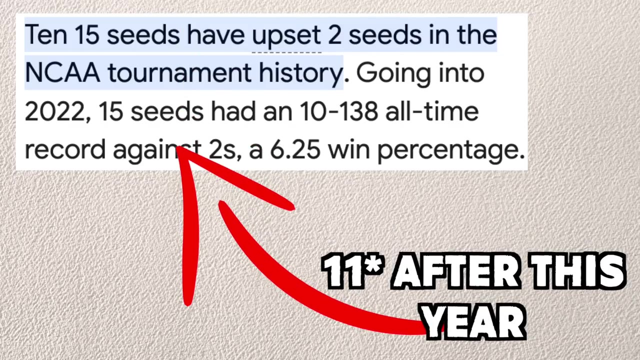 had 214 seeds in tournament. history, make the sweet 16 chattanooga in 1997 and cleveland state in 1986- and only 22- 14 seeds have ever won in march. madness when it comes to 15 seeds upsetting two seeds. we've seen it happen 11 times. a couple notable upsets: 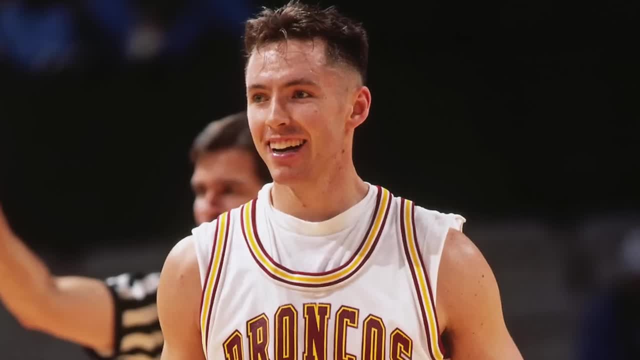 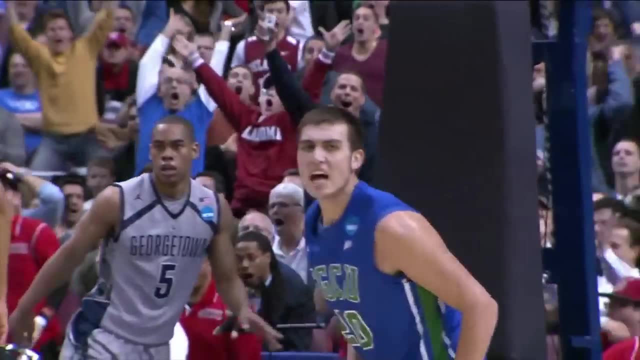 are cj mccollum and lehigh in 2012 and steve nash and santa clara in 1997. three other notable 15 seed runs are florida gulf coast, aka dunk city in 2016, one of the most fun mid-major teams of all time. 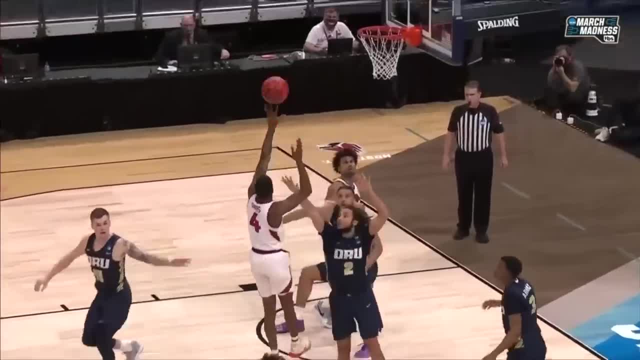 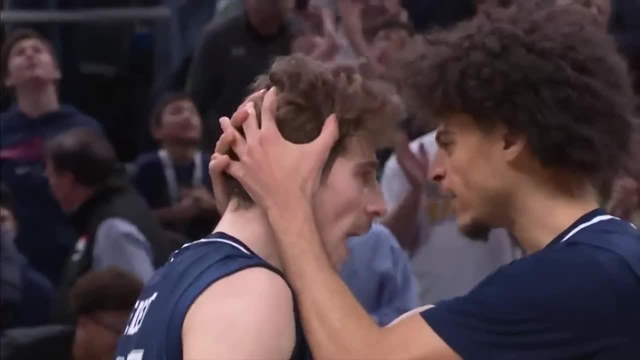 oral roberts in 2021. they actually almost made the elite eight, but lost on a last second shot versus the arkansas razorbacks and st peters just last year, who do have the record for the furthest a 15 seed has ever went in this tournament. what may be the most impressive thing about the? 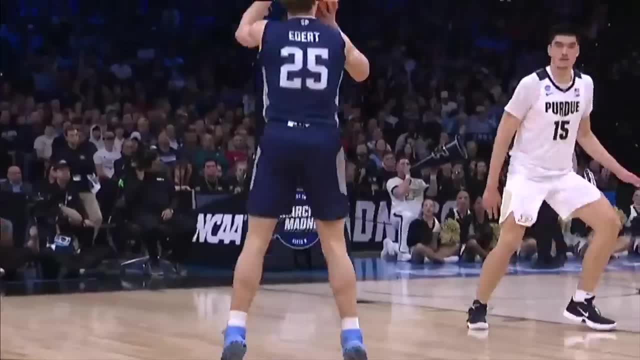 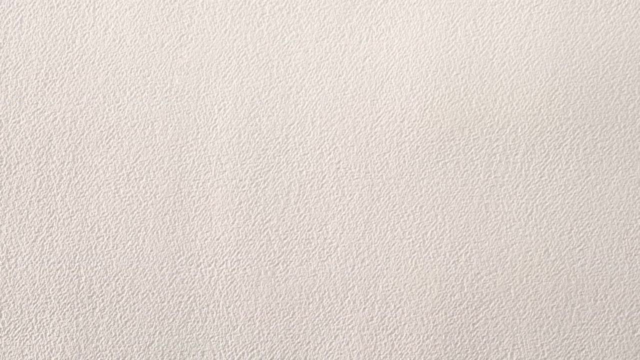 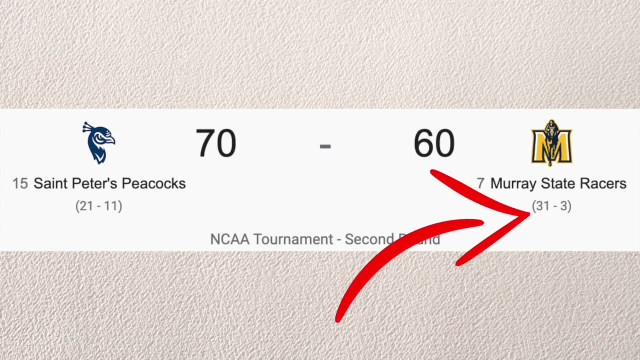 st peters run last year. all three of their wins were against very, very good teams. in the opening round they beat kentucky in overtime, 85 to 79, which had the national player of the year in oscar shibuya. in the second round they beat a murray state team that was 31 and 2 on the year. 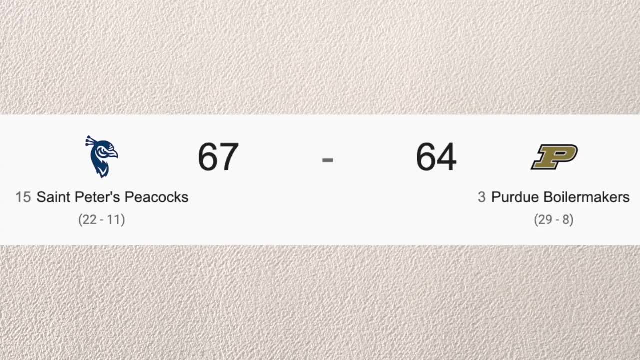 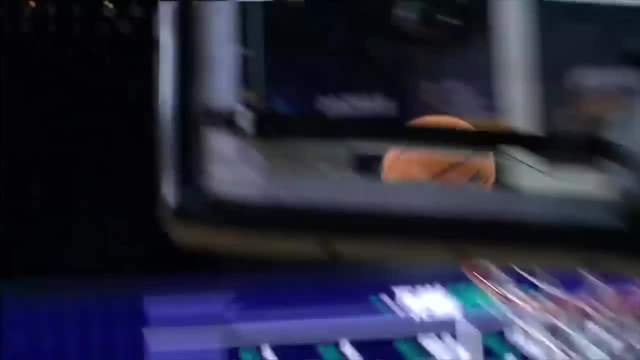 and finally, in the sweet 16, they beat a purdue team that had jayden ivy, the fifth overall pick in the 2022 draft. unfortunately, midnight finally came for the cinderella team losing by 20 points against the arkansas razorbacks and st peters run. last year, all three of their wins were against.